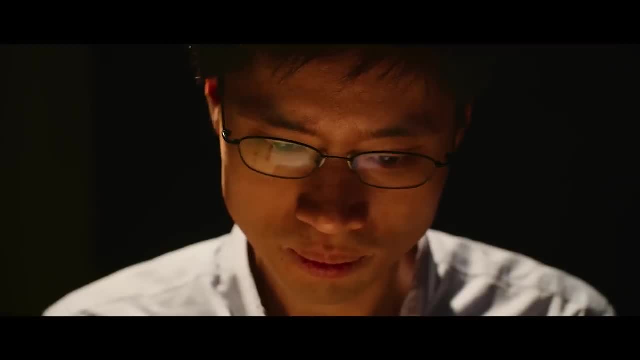 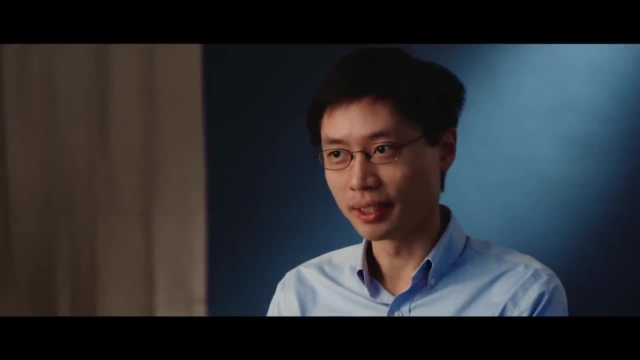 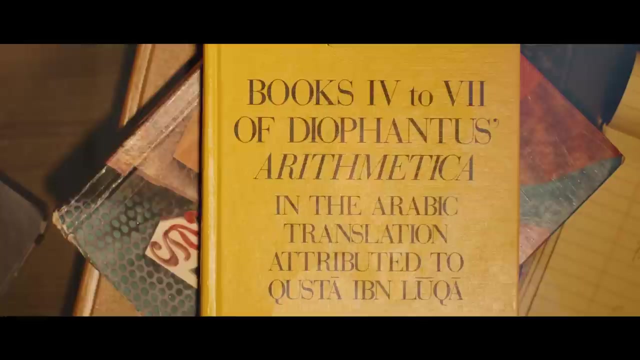 Diophantus of Al-Kharwizmi, the 15th century mathematicians, and the work of Indian mathematicians, And I found out that actually the key parts of this method had been discovered hundreds of years ago and thousands of years ago, and anyone could put them all together, This method. 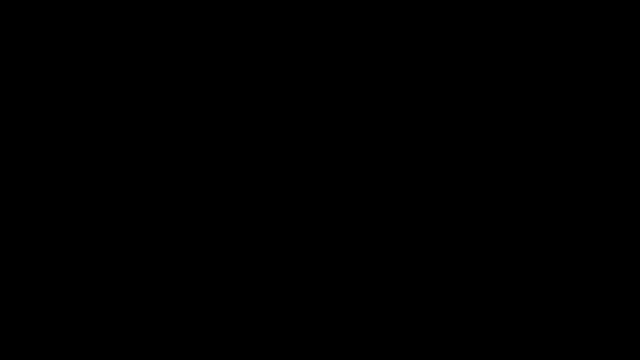 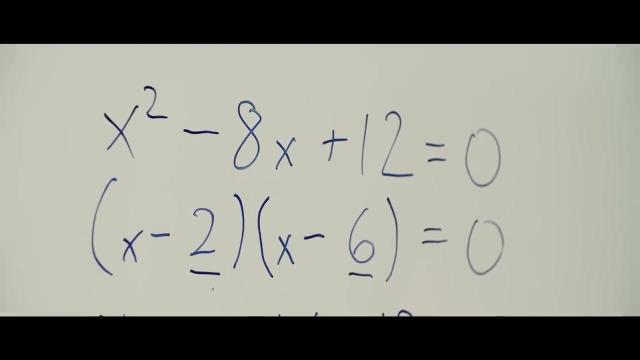 is direct and intuitive and lets you think through every step. Suppose you have a quadratic equation: x squared minus 8x plus 12 equals zero. Normally we, when we do a factoring problem, you're trying to find two numbers that multiply to 12 and 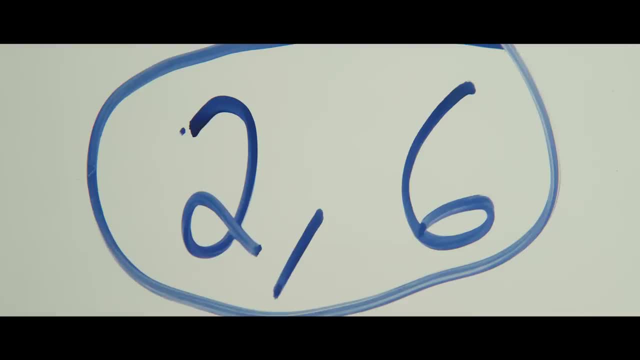 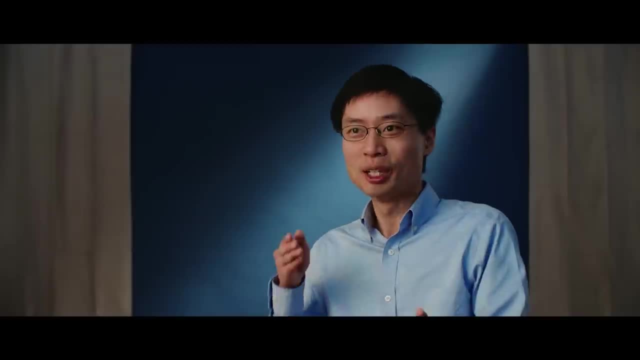 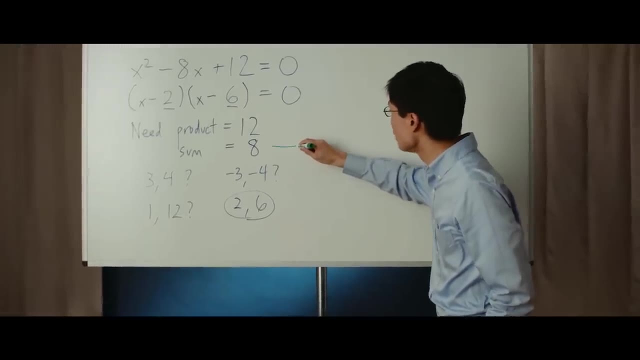 add to 8.. Those two numbers will be the solutions to the quadratic. Students spend a long time doing guess and check, which can be frustrating because one hopes that math gives a precise way of solving questions where you don't have to guess. Instead of starting from factoring the product, I start from the sum. If I have two numbers. 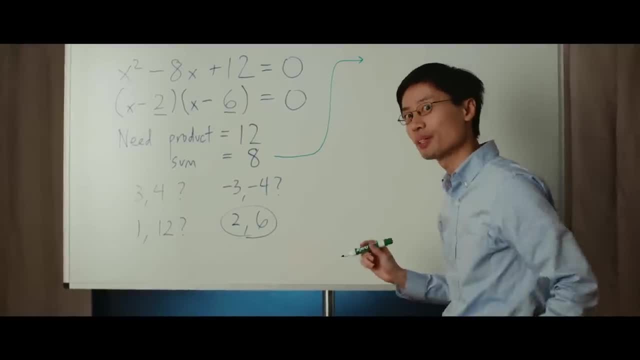 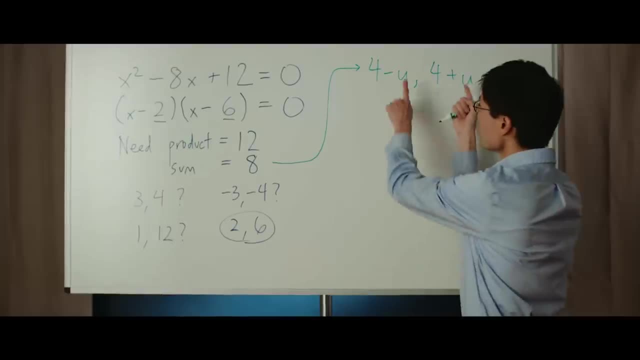 whose sum is 8, then they need to be the same distance away from their average. So the two numbers are 4 minus 8.. And 4 plus 8. for some unknown u, These two are supposed to multiply to 12.. But when you 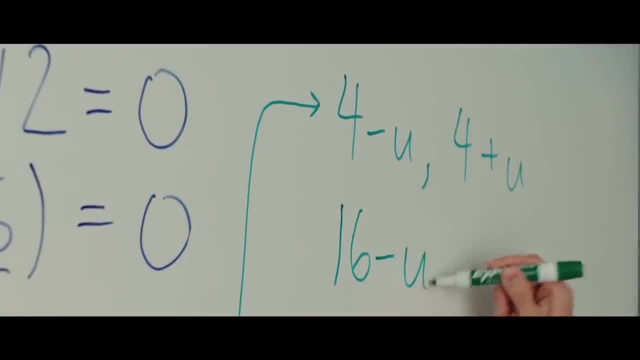 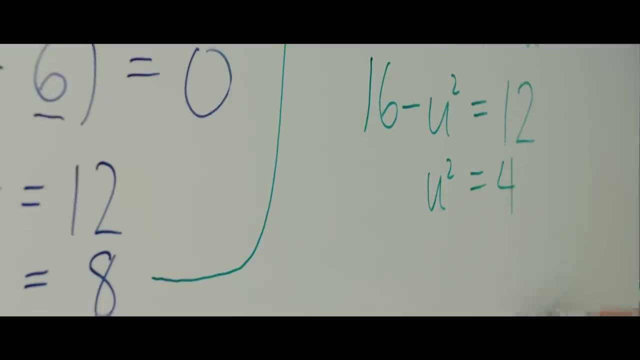 multiply this. it's beautiful. The middle terms cancel And I need to get a u so that 16 minus u squared is 12.. That comes when I find a u squared to be 4.. And that comes when I have a u which is either plus or minus 2.. Whichever one of those you take up there, 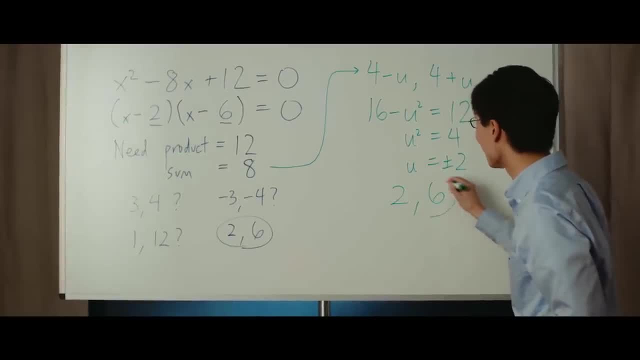 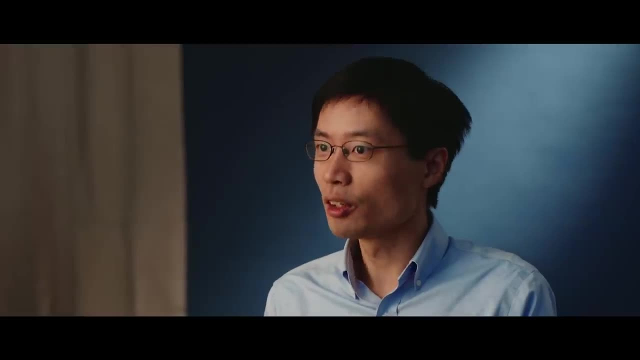 you will get that the two numbers are 2 and 6. And those are the two numbers that are the same. Add to 8 and multiply to 12, with no guessing, Because this method solves the problem by starting from the sum it can be used to solve. 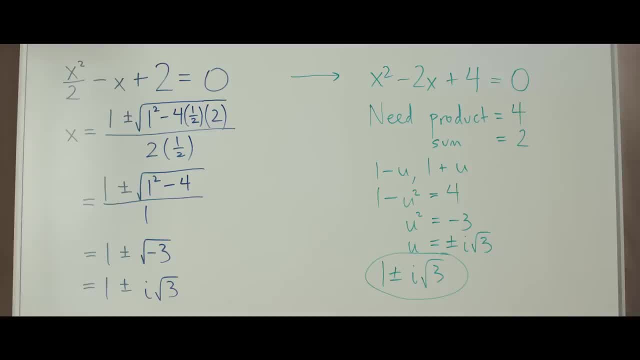 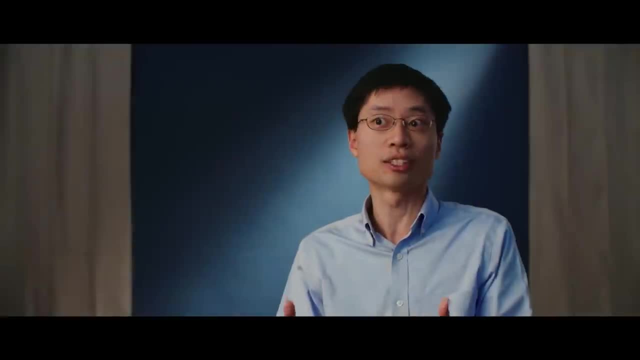 any quadratic equation. I wanted to share it as widely as possible with the world because it can demystify a complicated part of math that makes many people maybe feel like math is not for them. I think that if one can show that mathematics is actually a subject, that's 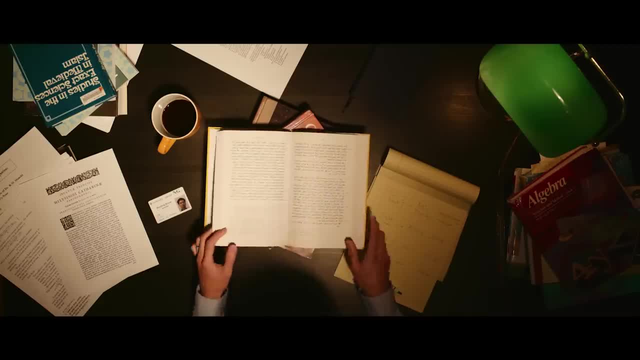 still alive in a way that every single person can appreciate. this is a benefit, And the hope is that by getting this problem solved, we can solve any quadratic equation, And that's what I'm trying to do, And that's what I'm trying to do.